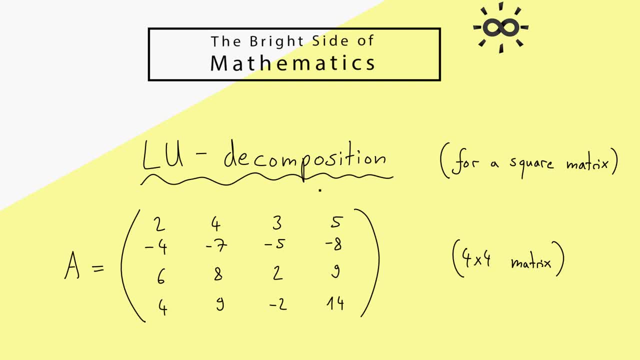 immediately tell you that doing the LU decomposition is basically just an expanded Gaussian elimination. Therefore, please remember, you can do the Gaussian elimination by just using row operations And what you get out is an upper triangular matrix in the end, And this is exactly the? U in our LU decomposition. 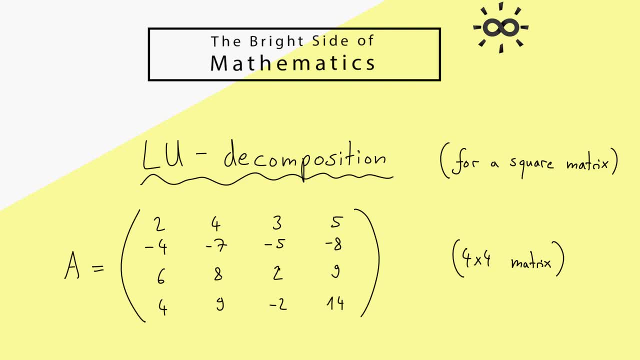 At this point I can give you a warning: We will not use row exchanges in this example here. Indeed, it's essential for the LU decomposition that you don't use row exchanges while applying the algorithm. This means that if you have a matrix where you really need row exchanges, 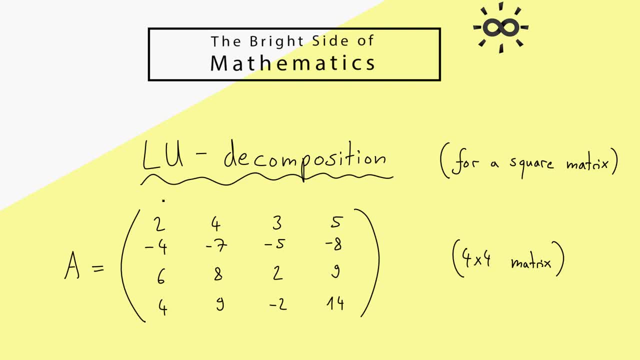 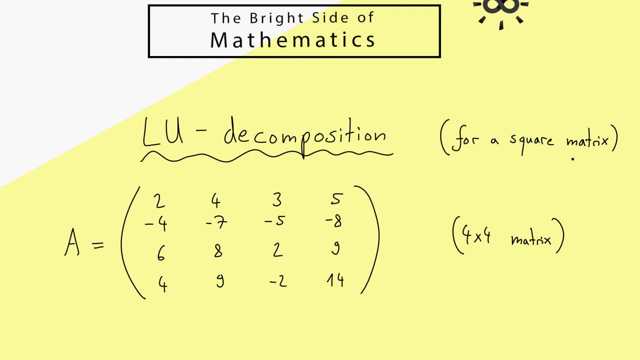 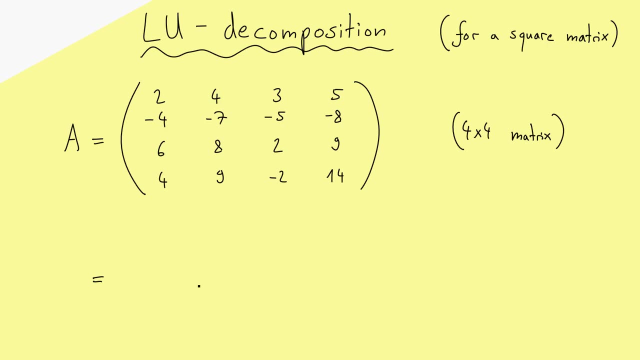 in the Gaussian elimination, then you should apply these all before hand and then just use the algorithm I now show you. Ok, then I would say we start with our nice example. here. The first step is always to include an identity matrix with the right size. Here it will be. 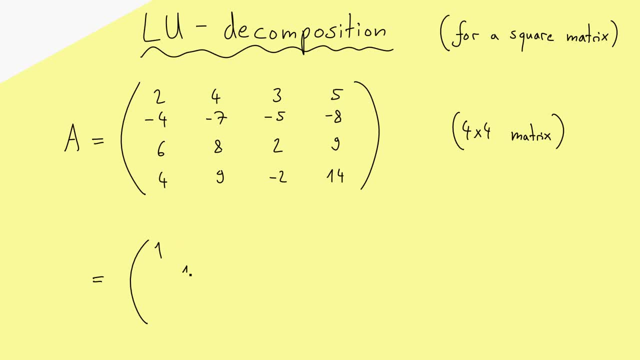 4x4 matrix. so I use 1,, 1,, 1, 1 on the diagonal and the rest are zeros, And on the right hand side I just copy my matrix from before. Obviously the equality still holds because we just multiplied the identity matrix. 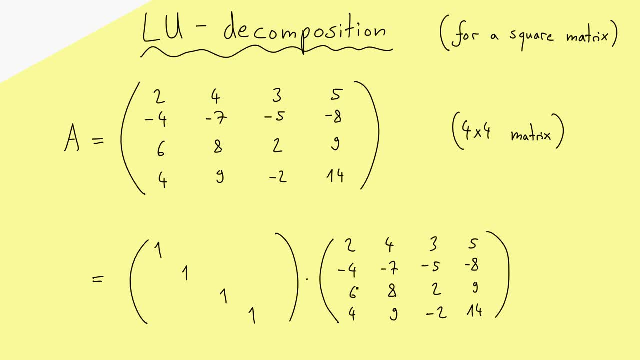 And now you see we almost have our LU decomposition here. We will transform the identity matrix into a lower triangular matrix, So we will fill in numbers here but not here, and we will transform this one to an upper triangular matrix. This means that we now just use the normal Gaussian elimination. 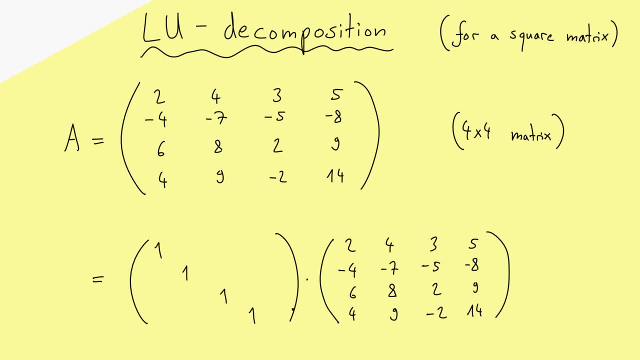 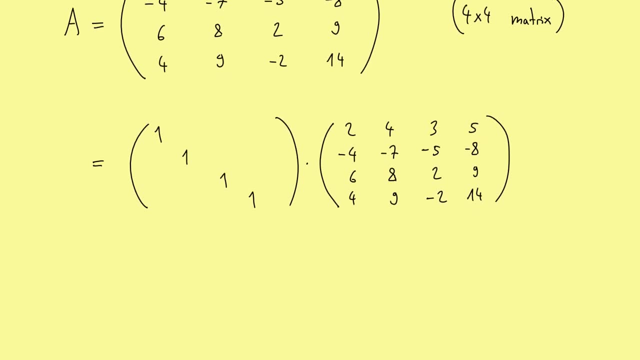 on the right, but now we also memorize all the steps with the help of the matrix on the left. Okay, you will see immediately how this works with the first step. Okay, so i copied the first row because we won't change it, but we will change all the other rows. 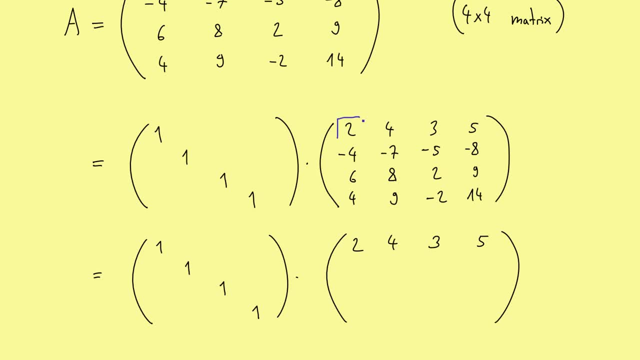 Now in the first Gaussian elimination step, we use this number as a pivot and we want to generate zeros below it. Therefore, to get a zero here in the second row, we have to use 2 times the first row. Hence we can write this as use the second row. 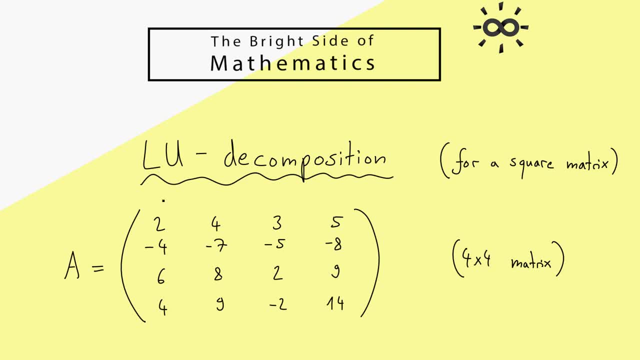 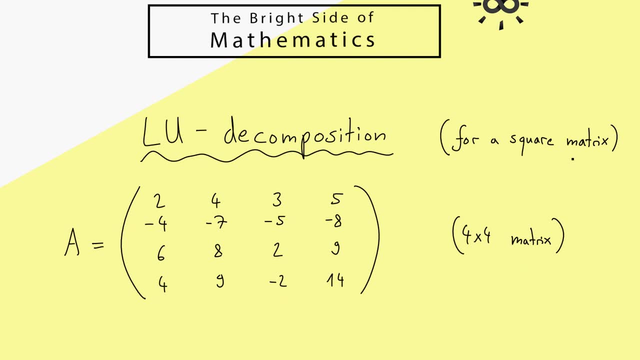 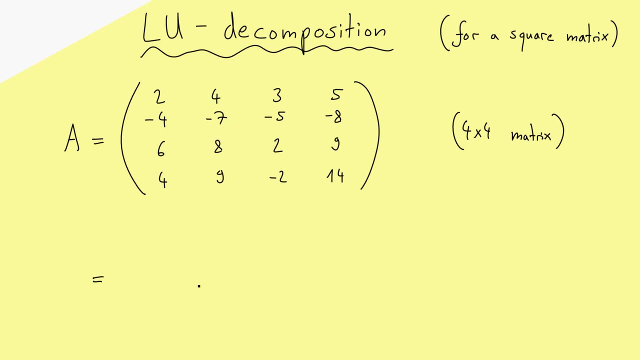 in the Gaussian elimination, then you should apply these all beforehand and then just use the algorithm I now show you. Ok, then I would say we start with our nice example here. The first step is always to include an identity matrix with the right size. Here it would be a: 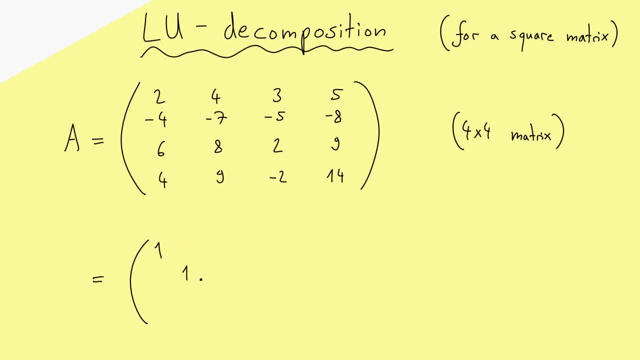 4x4 matrix. so I use 1,, 1,, 1, 1 on the diagonal and the rest are zeros, And on the right hand side I just copy my matrix. Obviously the equality still holds because we just multiplied the identity matrix. 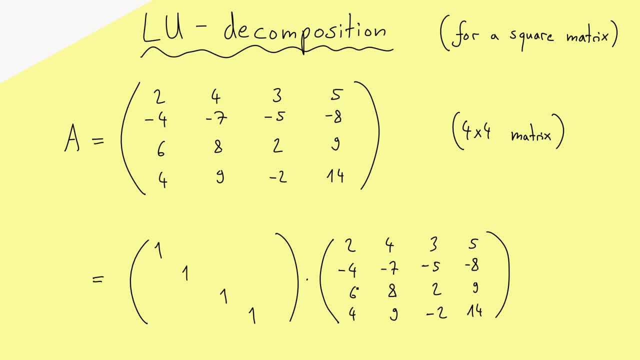 And now you see we almost have our LU decomposition here. We will transform the identity matrix into a lower triangular matrix, So we will fill in numbers here but not here, And we will transform this one to an upper triangular matrix. This means that we now just use the normal Gaussian elimination on the right. 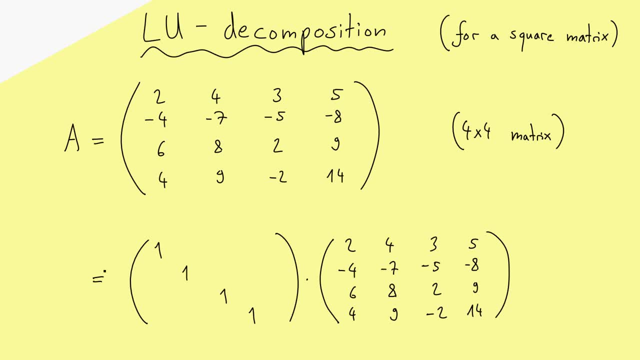 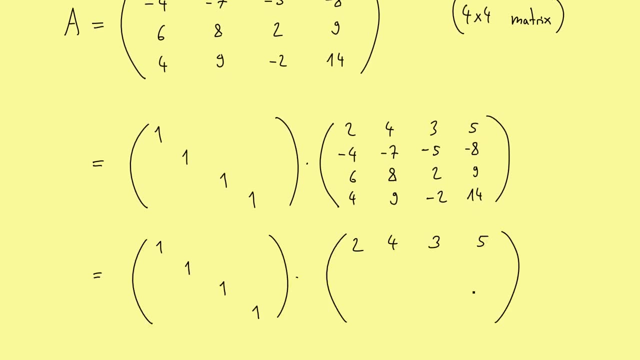 But now we also memorize all the steps with the help of the matrix on the left. Ok, you will see immediately how this works with the first step. Ok, so I copied the first row because we won't change it, but we will change all the other rows. 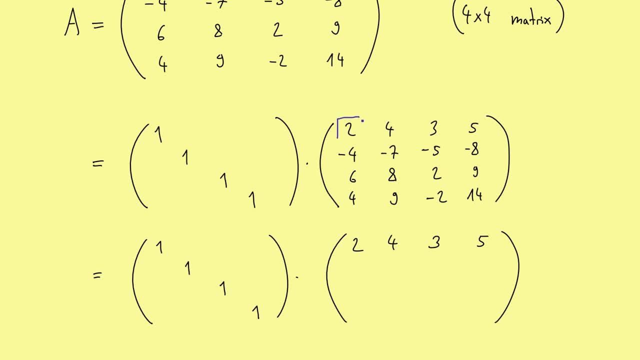 Now on the first Gaussian elimination step. we use this number as a pivot and we want to generate zeros below it. Therefore, to get a zero here in the second row we have to use the first row as a positive. So we use 2x the first row. 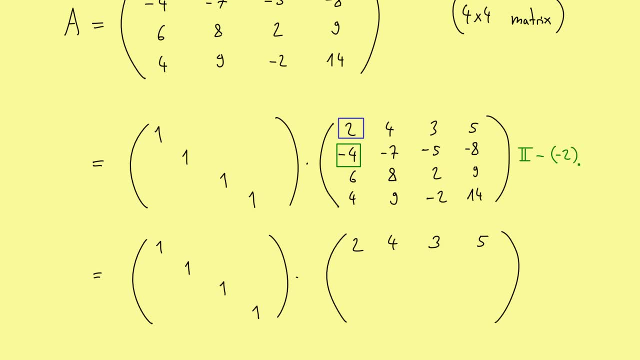 Hence we can write this as: use the second row minus minus 2x the first row. Of course we could rewrite this as plus 2x the first row, but for the LU decomposition it's always helpful to use a minus sign here. This means that we always subtract multiples of another row. 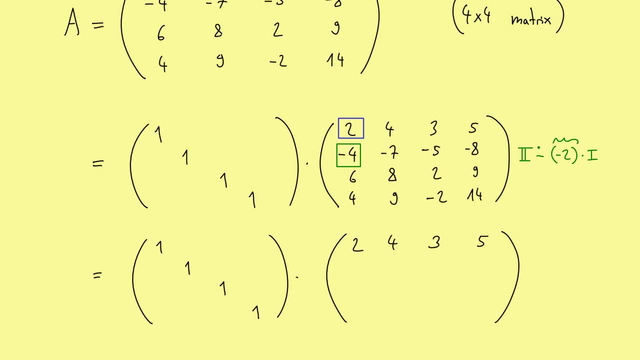 This number here we subtract, is the number we will put in the matrix L. Where to put it? is very easy, because here we generated a zero And at the exact same position we put the new number in the matrix L, And in the same way it works for all other positions here. 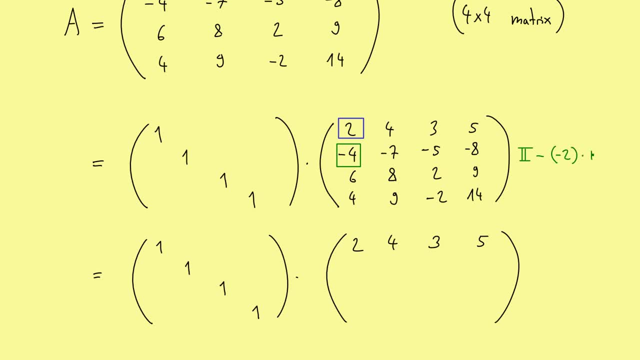 minus minus 2 times the first row. Of course, we could rewrite this as plus 2 times the first row, but for the LU decomposition it's always helpful to use a minus sign here. This means that we always subtract multiples of another row. This is very helpful because 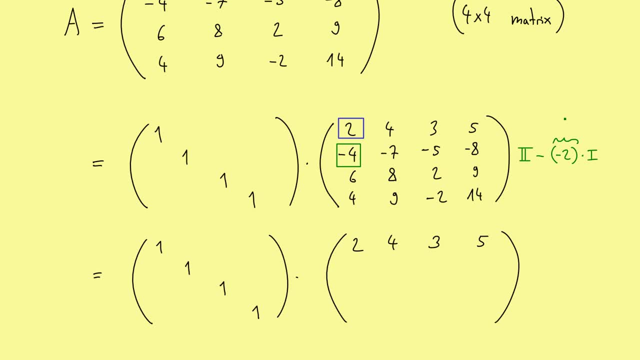 this number here we subtract, is the number we will put in the matrix L. Where to put it? is very easy, because here we generated a zero and at the exact same position we put the new number in the matrix L, And in the same way it works for all other positions here. 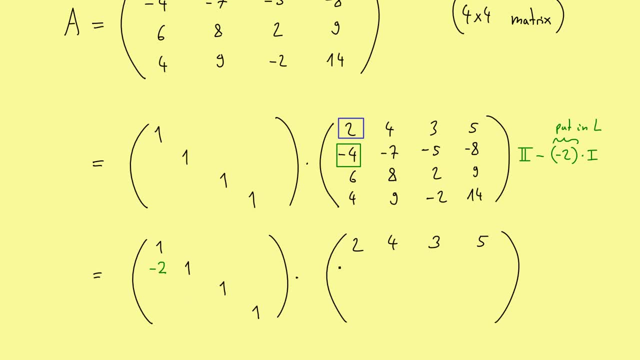 Now with the matrix multiplication, you see that this is indeed the correct sign we chose, because if you multiply 2 with our minus 2 here, you get out indeed to minus 4, as we want. However, still we have to do our calculation here, so we do our Gaussian elimination step. 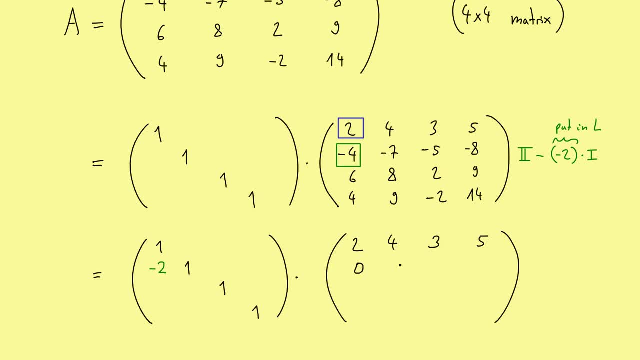 which means we have the zero here, as wanted, Here we have 1, here we have also 1 and there we have 2.. Ok, now we can do the same thing for the third row, which means we take the third row and we have to subtract a multiple of the first. 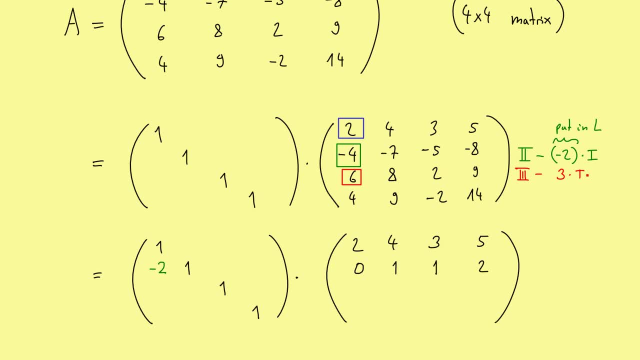 Which is here just 3 times the first row. Ok, now you know the multiple we subtract, so 3 is the number we put at the right position here. And of course we also have to do the calculation, which is 0 here minus 4, minus 7 and minus. 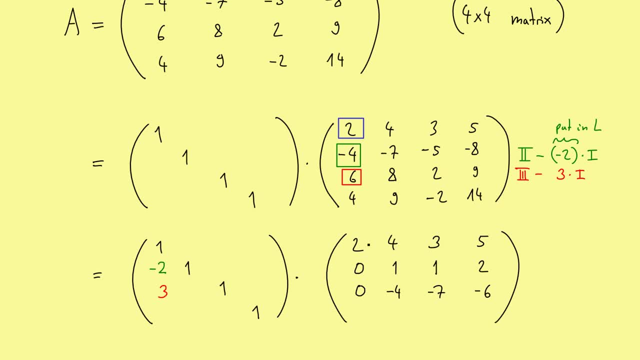 6. here Again we can check that our sign was correct. so if you multiply this column with this row, we get out 2 times 2.. So our 6.. And finally, we can do the whole thing for the last row. So I take the fourth row and I look at the multiple of the first row. I have to subtract. 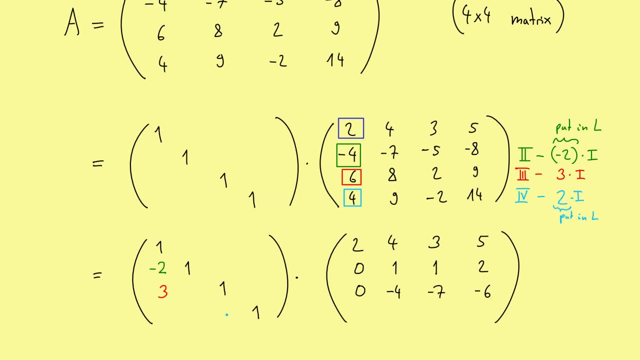 And here it is 2 times the first row. And now you already know we have to put this 2 into our matrix L, And also the calculation in the last row is not so hard. We have the zero here, Here we have 8.. 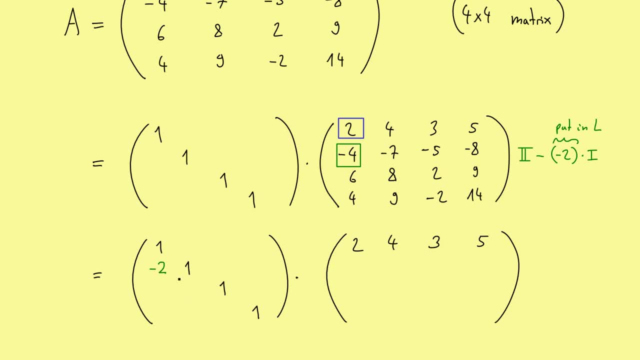 Now with the matrix multiplication, you see that this is indeed the correct sign we chose, Because if you multiply 2 with a minus 2 here, you get out indeed to minus 4, as we want. However, still we have to do our calculation here, So we do our Gaussian elimination step. 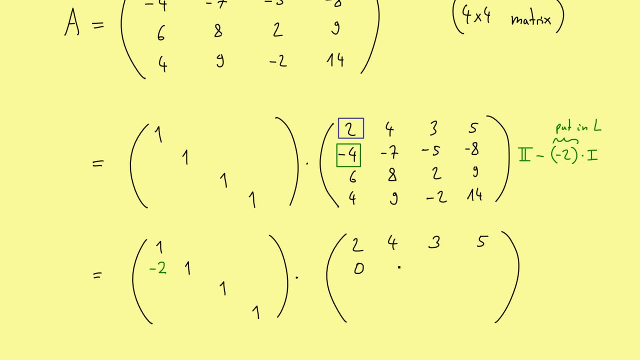 Which means we have the zero here, as wanted, Here we have 1.. Here we have also 1. And there we have 2.. Okay, now we can do the same thing for the third row, Which means we take the third row and we have to subtract a multiple of the first row. 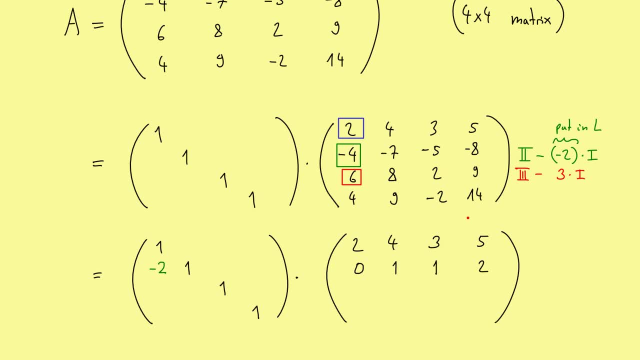 Which is here Just 3 times the first row. Okay, now you know the multiple we subtract, So 3 is the number we put at the right position here, And of course we also have to do the calculation, Which is 0 here. 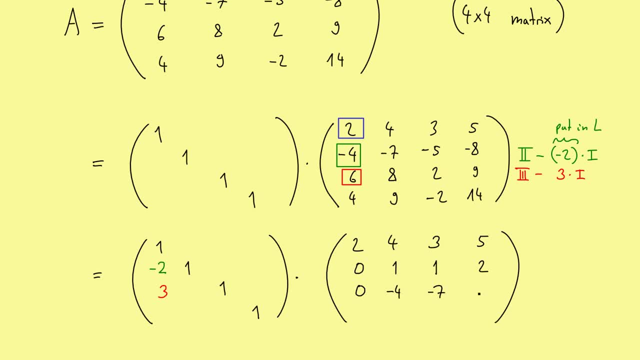 Minus 4.. Minus 7. And minus 6. here Again we can check that our sign was correct. So if you multiply this column with this row, we get out 2 times 3.. So our 6.. And finally, we can do the whole thing for the last row. 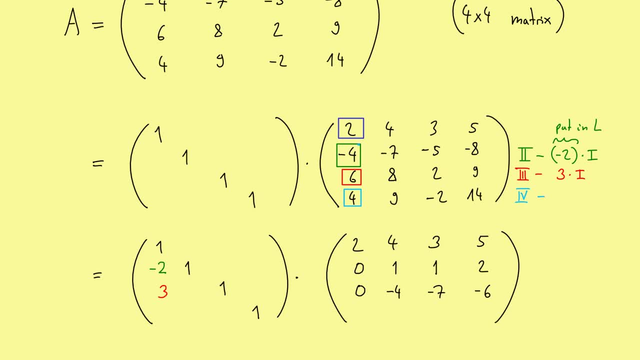 So I take the fourth row and I look at the multiple of the first row. I have to subtract And here it is 2 times the first row. And now you already know we have to put this 2 into our matrix L. And also the calculation in the last row is not so hard. We have the 0 here, here we have 8.. So 1 remains. 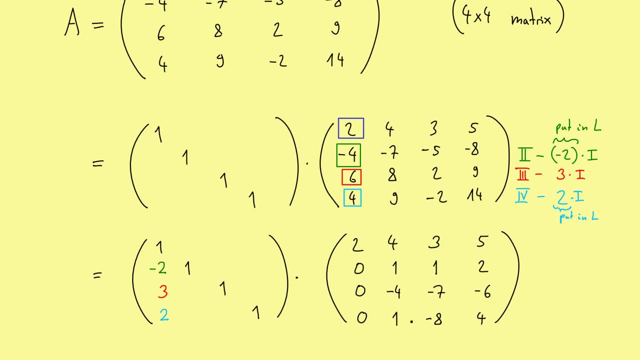 And here we have minus 8.. there four. Well, now we are finished with our first column, because everything is zero here. Now we go to our next column, so the second column, which means this is our new pivot. So the procedure would be exactly the same. we now just produce the 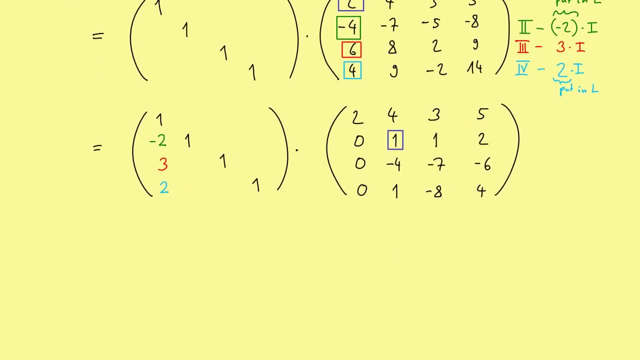 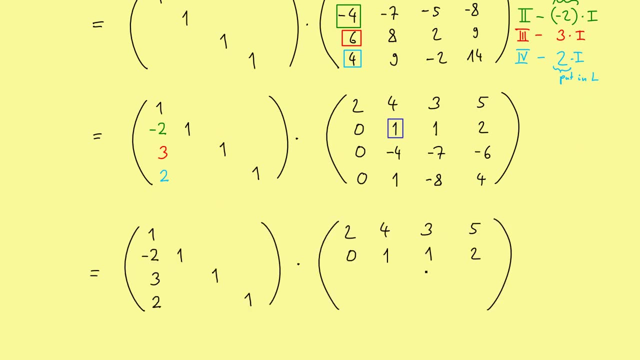 zeros here. Okay, in order to do this, let's start a new line, So let's copy everything and then do the same Gaussian elimination as before. We can copy the first two rows, because we won't change them anymore. The first step, of course, is to: 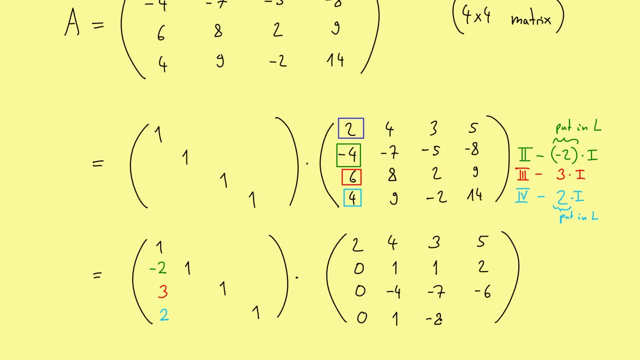 So 1 remains, And here we have 2.. And here we have minus 8 and there 4.. Well, now we are finished with our first column, because everything is zero here. Now we go to our next column, so the second column, which means this is our new pivot. 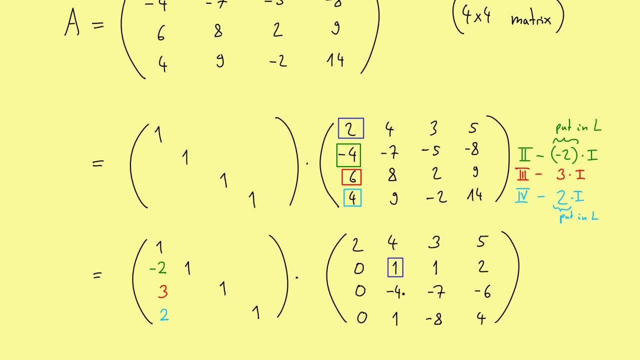 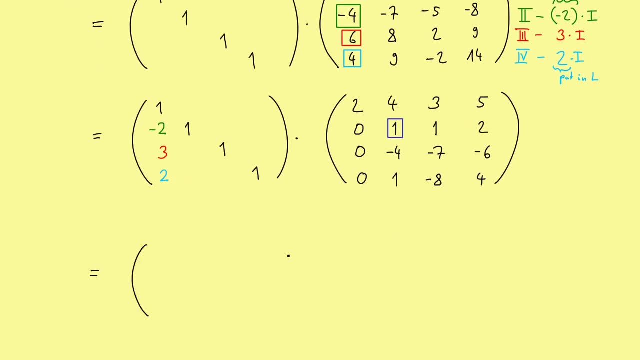 So the procedure would be exactly the same. we now just produce the zeros here. Ok, in order to do this, let's start a new line. So let's copy everything and then do the same Gaussian elimination as before. We can copy the first two rows because we won't change them anymore. 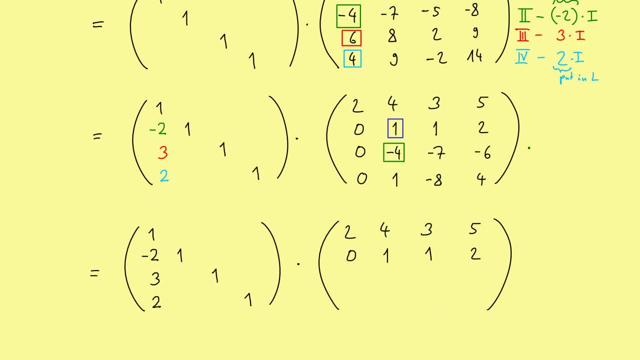 The first step is, of course, to generate a zero here, Which means that we take the third row and use the second row to change it. Now, you see, we have to add 4 times the second row to get a zero here, And therefore we write it as subtracting minus 4 times the second row. 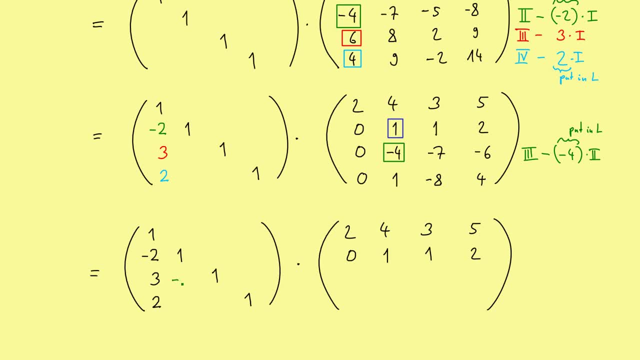 And now this multiple is the number we put here, And now we have to add 4 times the second row to get a zero here, And therefore we write it as subtracting minus 4 times the second row. So we put here at the right position. 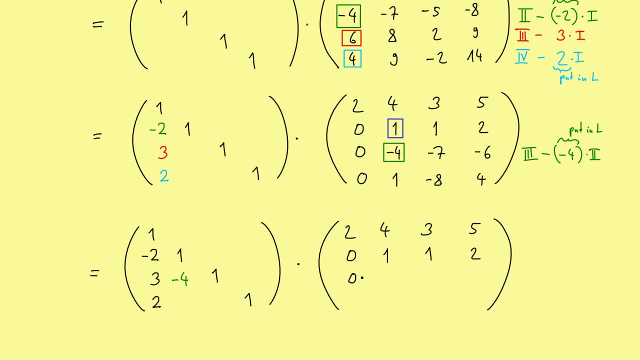 minus 4.. And our calculation in the third row gives us here zero, zero. Here we have 4 and minus 7, so minus 3.. and here we have 2.. Ok, so let's do the next step, which means generate a zero here. 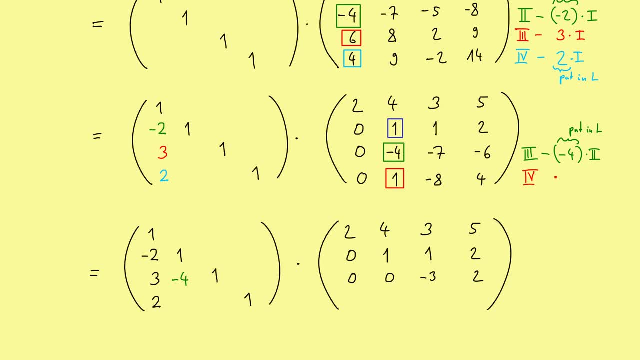 So take the fourth row and subtract the second row, So minus 1 times the second row. Again, this 1 is the thing we talked about. now put here in our matrix L, And the last calculation here is very easy: We just have 0, 0, minus 9,. 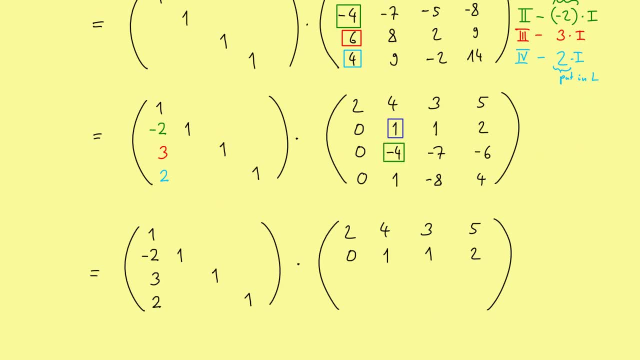 generate a zero here, Which means that we take the third row and use the second row to change it. Now, you see, we have to add four times the second row to get a zero here, And therefore we write it as subtracting minus four times the second. 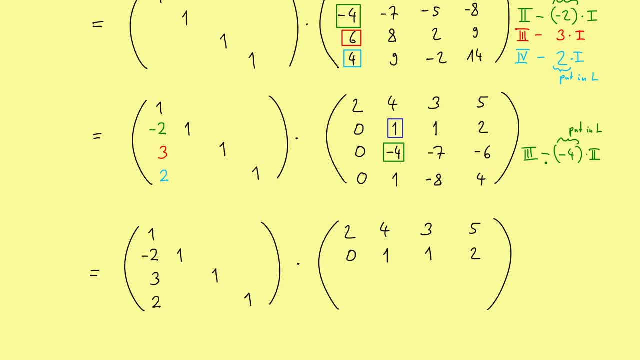 row. And now this multiple is the number we put here as a positive, the right position, minus 4.. And our calculation in the third row gives us here 0, 0.. Here we have 4 and minus 7, so minus 3, and here we have 2.. Okay so, 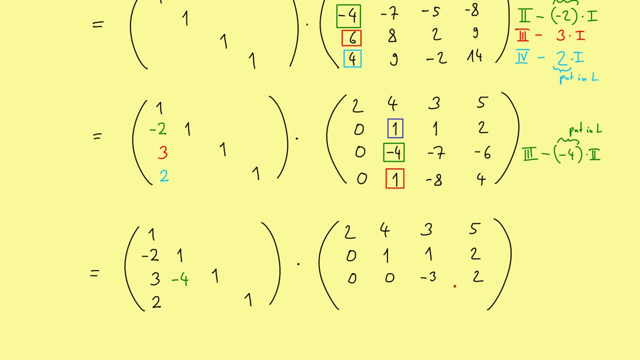 let's do the next step, which means generate a zero here. So take the fourth row and subtract the second row, So minus 1 times the second row. And again, this 1 is the thing we put here in our matrix L, And the last calculation here is very. 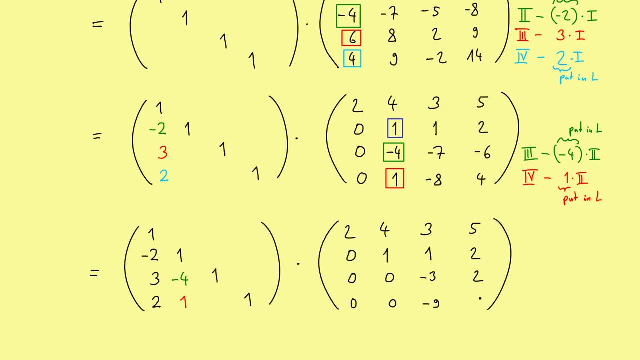 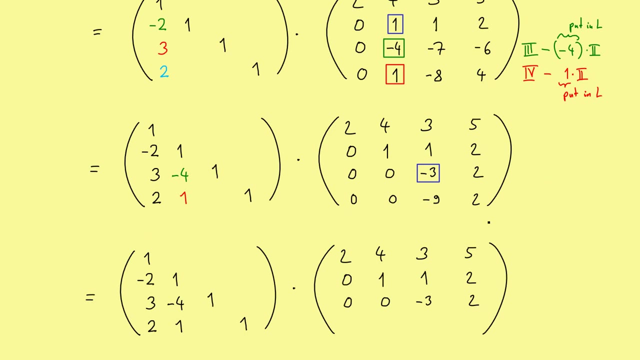 easy. We just have 0, 0, minus 9 and 2.. Okay, very good. So now you see, we just need one last step in our Gaussian elimination. So let's do that very quickly now. Well, I copied everything again except the last row, because this: 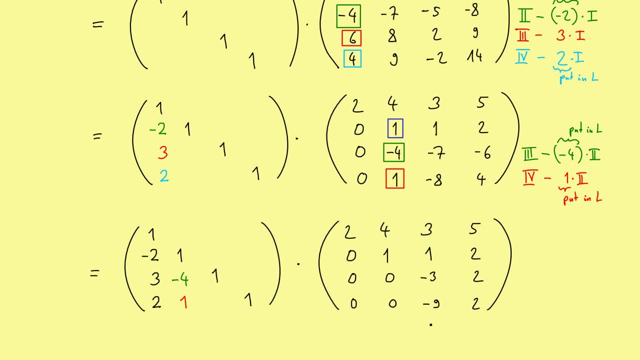 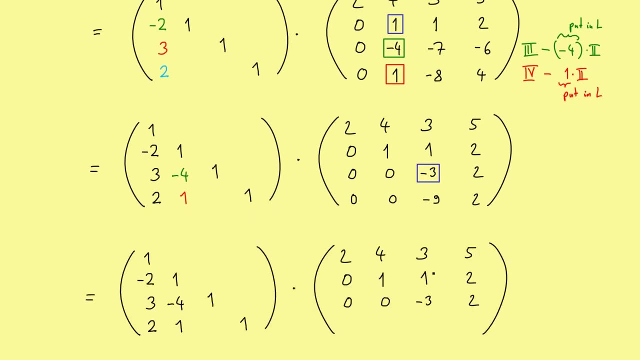 and 2.. Okay, very good. So now you see, we just need one last step in our Gaussian elimination. So let's do that very quickly now. Well, I copied everything again, except the last row, because this is the only one we change now, And you immediately see what we need. We just have to change the fourth. 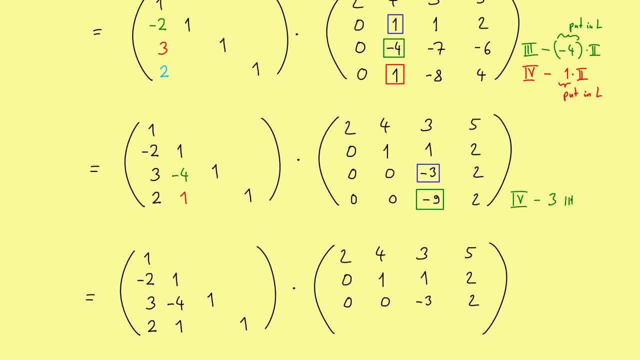 row by subtracting 3 times the third row And, as before, the number we subtract is the number we put in here. Then we just have the 0s here and minus 4 here, And there you have it, That's our. 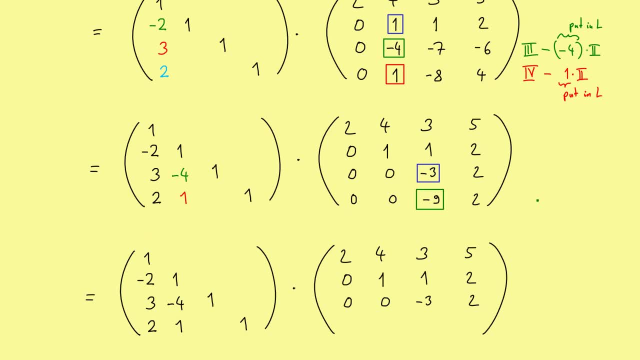 is the only one we change now And you immediately see what we need. We just have to change the fourth row by 1. Subtracting 3 times the third row And, as before, the number we subtract is the number we put in here. Then we just have the zeros here and minus 4 here, And 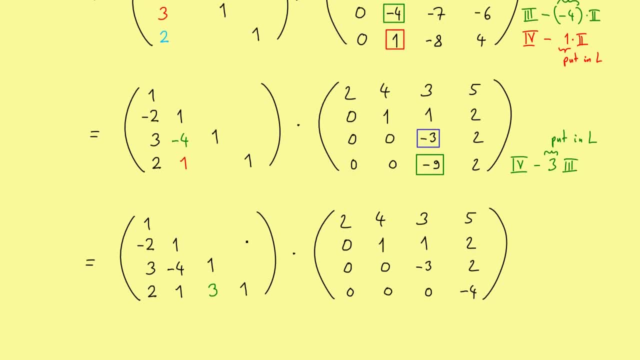 there you have it. That's our LU decomposition. On the left, we have our lower triangular matrix, which we call L, And we want to choose it with only ones on the diagonal. And you see, that is exactly what we get out with this algorithm. 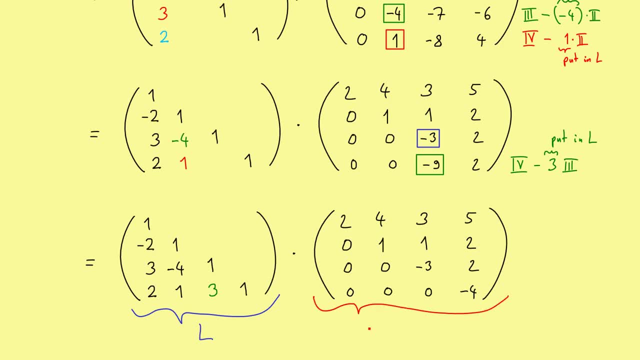 And on the right hand side you see, this is our upper triangular matrix U. There, on the diagonal, everything can happen. Now please recall that you get U by just using Gaussian elimination and L by saving all the steps in the Gaussian elimination. Therefore, the matrix multiplication here gives us in fact our